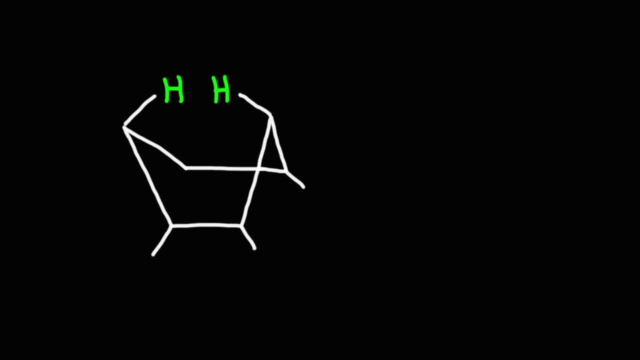 And then let's show the other hydrogen atoms, So the hydrogen atoms in red, they're eclipsed with the ones in blue. And let's draw the other hydrogen atoms next to the flagpole ones, So that's a decent representation of the bow conformation. 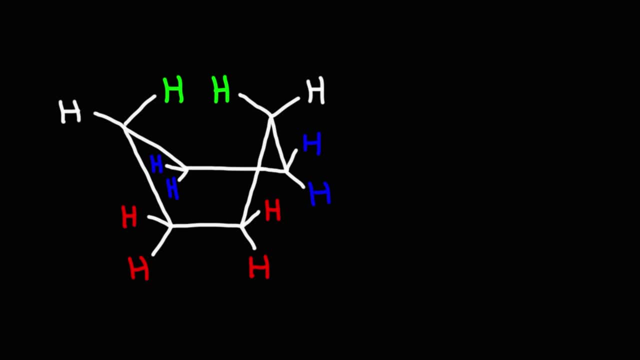 Now what you need to know is that the bow conformation is relatively unstable relative to the other three conformations. On a test, you need to know that the half chair is the least stable conformation. Let me put this in a smaller font. 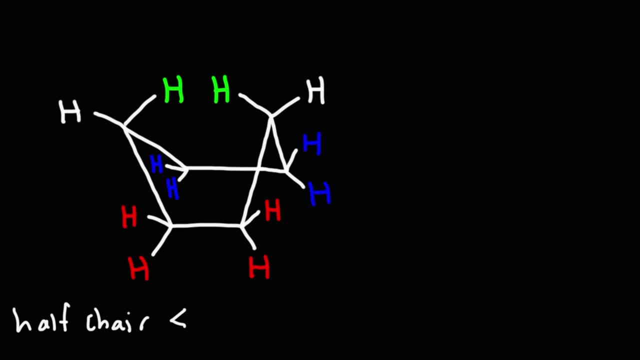 After the half chair conformation, next is the bow conformation. The twist bow conformation is slightly more stable than the bow And the most stable is the chair conformation, But the focus of this video is the bow conformation. So why is the bow conformation less stable than the twist bow and the chair conformation? 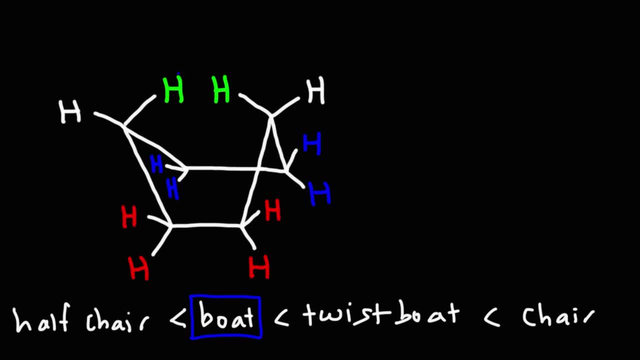 One of the reasons is due to the flagpole hydrogen atoms. As you can see, they're pretty close, And so you're going to have some steric strain. The steric strain is due to the electron repulsion that occurs when the hydrogen atoms get close to each other. 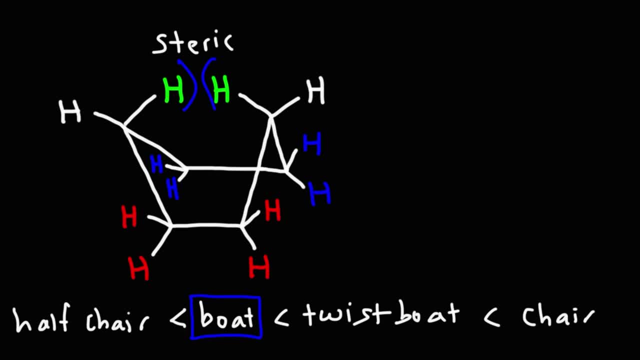 As their electron clouds approach each other, you're going to have electron repulsion. Now the bow conformation also has torsional strain. If we focus on the CH bonds on adjacent carbons, notice that these two hydrogen atoms, they're clips to each other. 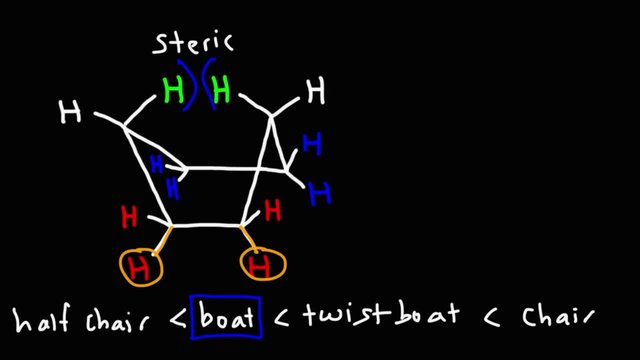 And torsional strain occurs among atoms that are about within three bonds apart. So one, two, three. So any time you have atoms that are eclipse with each other, and if they're within three bonds apart, you're going to have torsional strain. 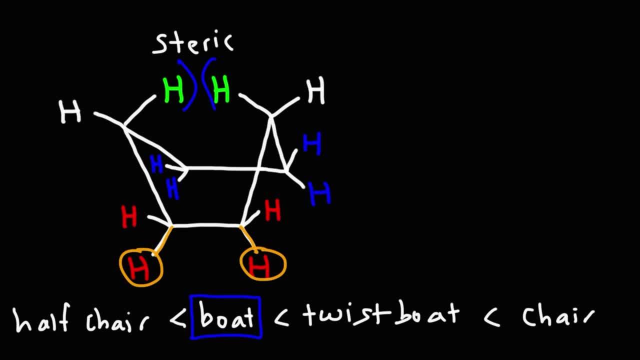 Now, if we were to take the bulk conformation and if we were to twist it- let's turn this side to the right and this side to the left- We can form the twist bulk conformation. In the twist bulk conformation, the flagpole hydrogen. 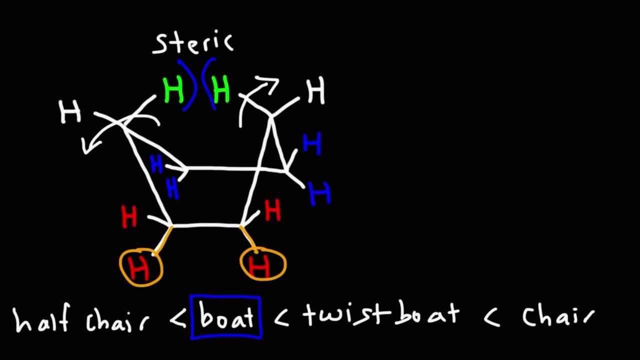 atoms have moved apart. As a result, a lot of the steric strain that was in the bulk conformation has been greatly reduced, and so we see that the twist bulk conformation is more stable than the bulk conformation, because we don't have the flagpole hydrogen atoms clashing into each other as we're doing in the 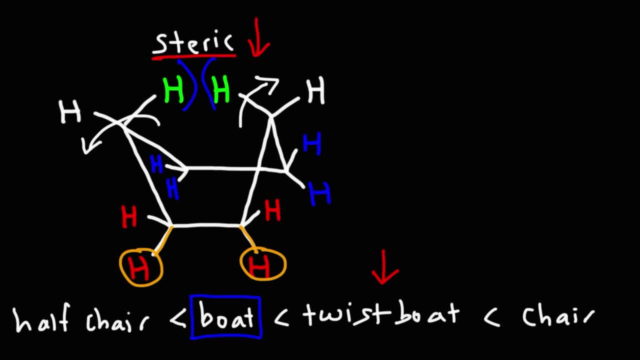 bulk conformation. So what you need to know about the bulk conformation is that it possesses steric strain due to the flagpole hydrogen atoms clashing to each other, and there's also some torsional strain among the CH bonds of eclipsen hydrogen atoms that are on adjacent carbons. The other thing you 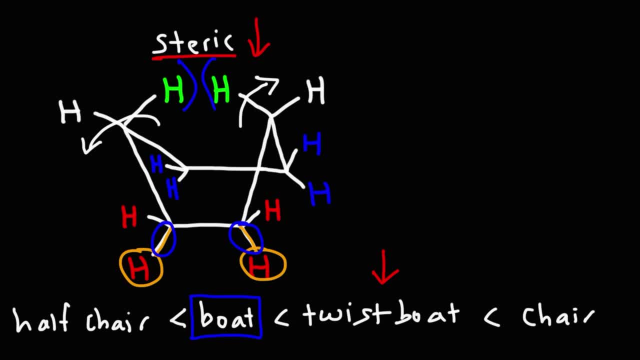 need to know is that the twist bulk is more stable than bulk conformation due to the fact that the flagpole hydrogen atoms. they're no longer clashing into each other as they were in the bulk conformation. so you need to throw all your the bowl conformation- And remember the half chair- is the least stable conformation and 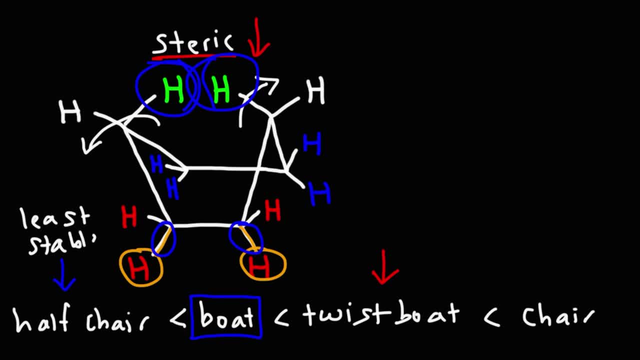 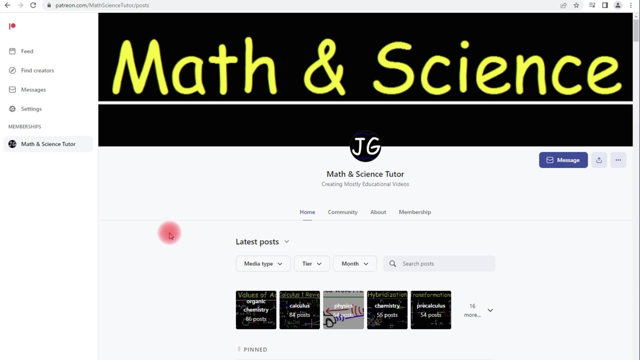 the chair conformation is the most stable conformation of cyclohexane. By the way, for those of you who want more practice problems on chair conformations, stuff like that, check out the links in the description section below this video. Now for those of you who want to access my extended organic chemistry videos, 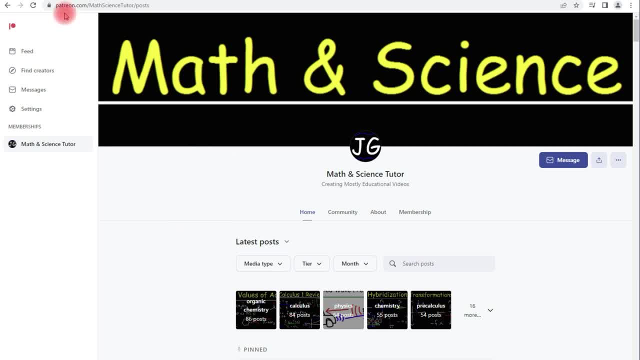 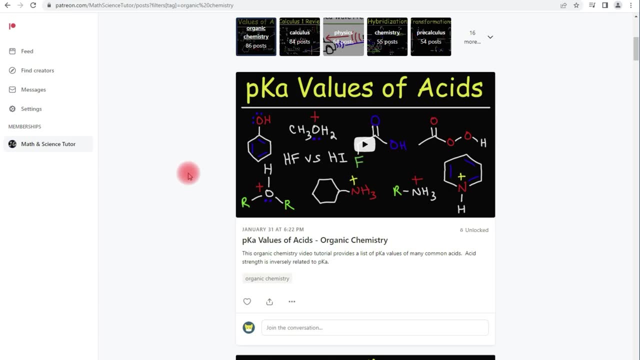 you can access it at my Patreon membership program at patreoncom slash math science tutor or in my YouTube membership program, which you can join in the video below. Now, if we click on this organic chemistry post, it'll show you all my full length organic. 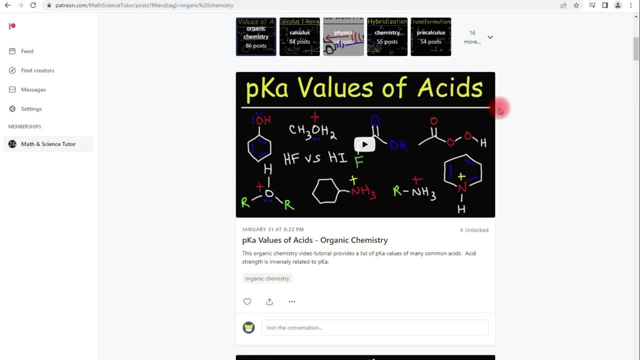 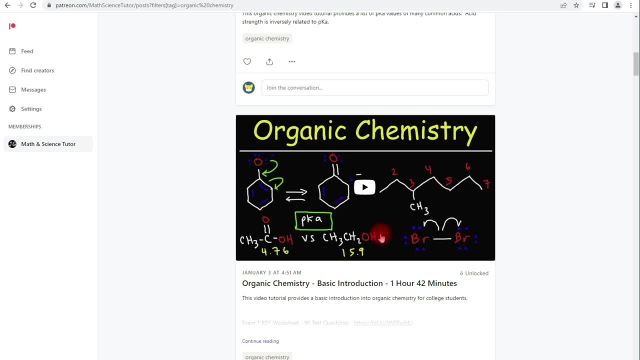 chemistry videos. So I have this video on pKa values for those of you who are studying acids and bases. For those of you who are just studying organic chemistry, this basic introduction video will really help you get started, And I have some other videos as well. 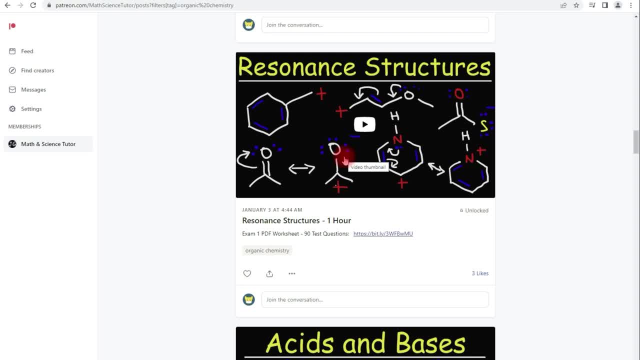 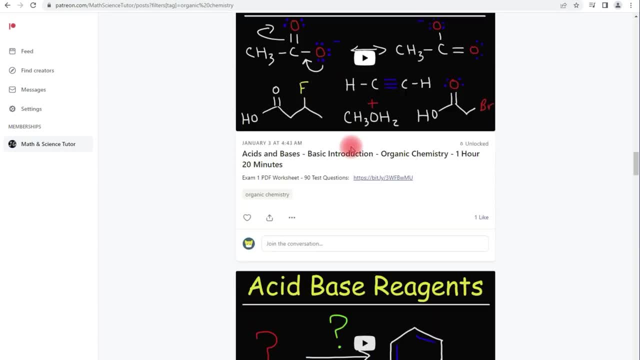 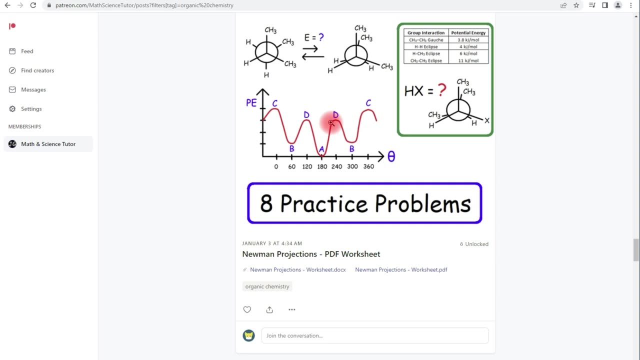 hybridization resonance structures. The free version of this video is about 20 minutes long on YouTube, but the full length version is about an hour long. Acids and bases- functional groups- Newman projections. The worksheet contains all of the problems in the full length video. 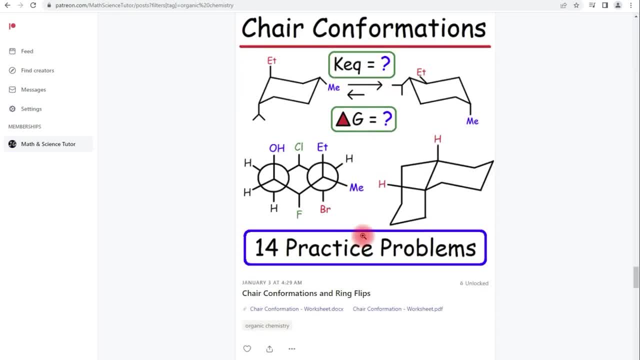 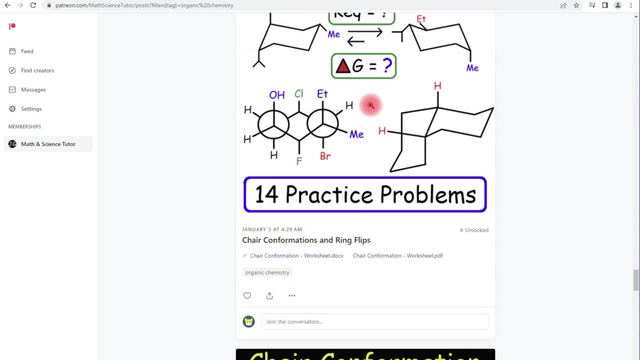 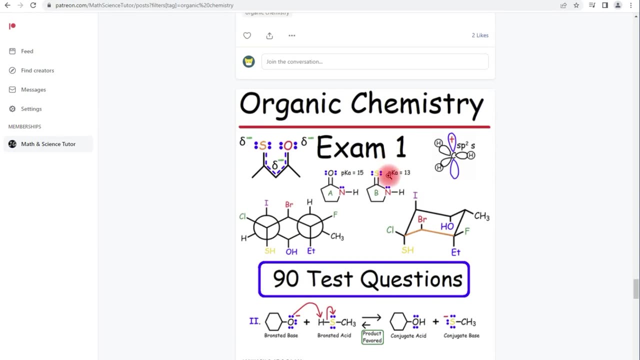 Some of you have asked for worksheets. You prefer to work through the problems that way instead of, you know, watching a long video. So I have it for, not all of my videos, but some of them. So we have chair conformations. Now for my organic chemistry exam, one video you may have to. 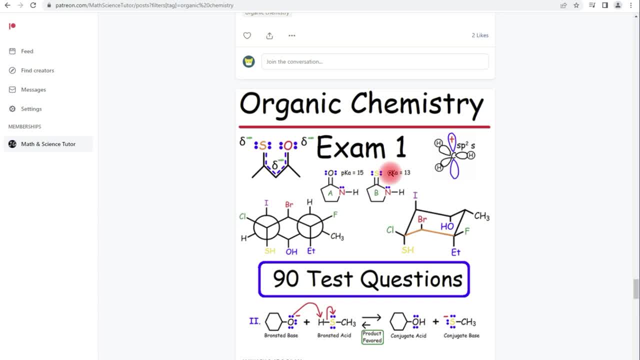 type it in in the search box to get it. Or if you look at the description section of the referring video, it'll show you all the problems in the full length video. So I have it for all of my videos. It'll take you directly to that link. But here is the worksheet Now. if you want to watch a seven. 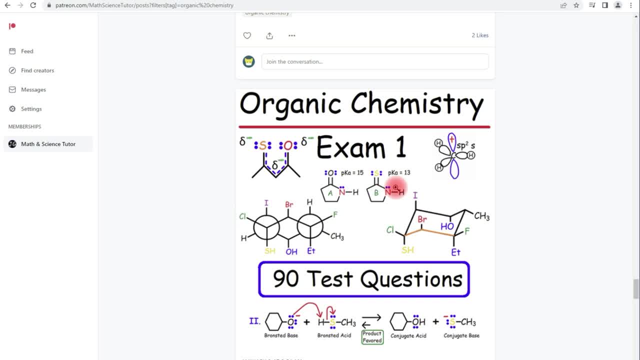 hour video. you can do it that way, But if you prefer to print out the worksheet and work through the problems that way, you could do that as well. By the way, post a comment in below this video. I want to know what your thoughts are. Do you prefer to watch the seven hour video or do you? 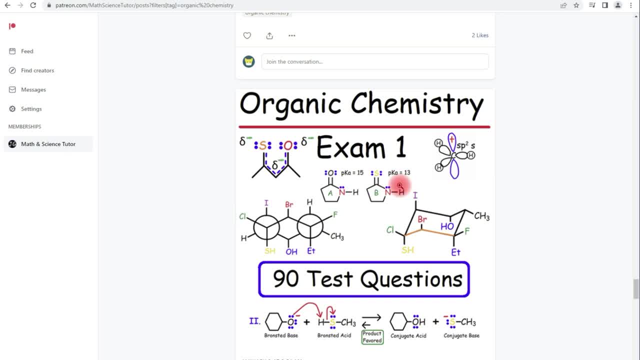 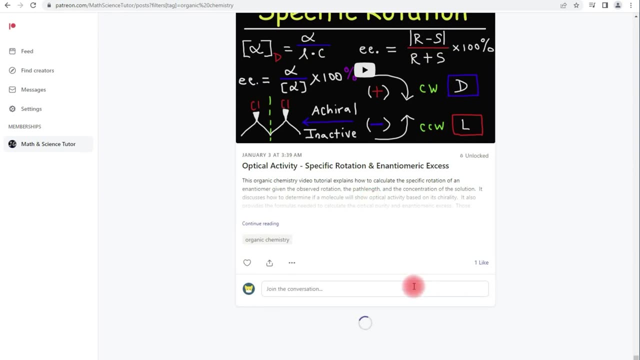 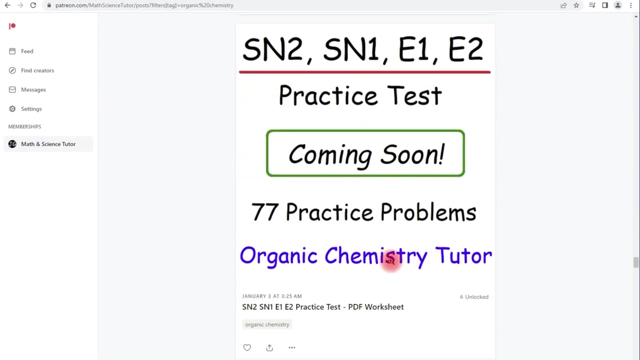 prefer to study for the exam by getting a printout of the worksheet And working through the problems while you're in school. Let me know in the comment section below. Now I have other videos. stereochemistry: specific rotation, SN1, SN2 reactions. There's a practice test on that, 77 practice problems. So here's the video. 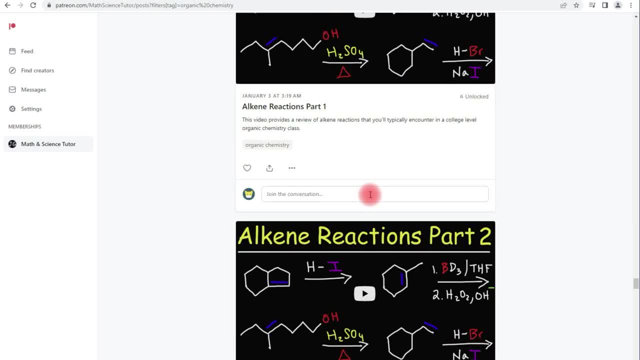 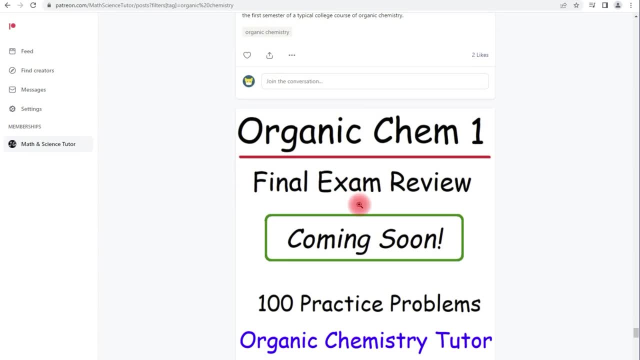 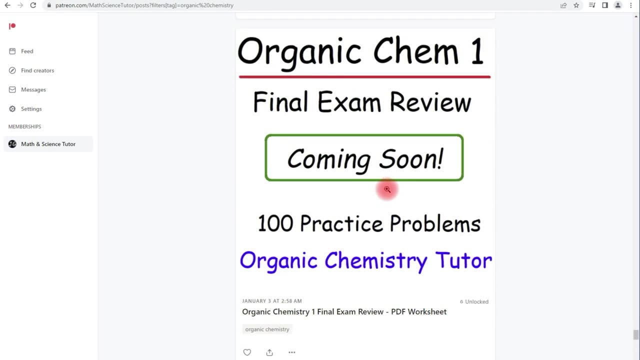 with the practice test, but I haven't done the worksheet yet. We got alkene reactions, alcohol reactions, radical reactions and then my organic chemistry- one final exam review video. So the video is actually finished, but the worksheet is coming soon, So let me know for.